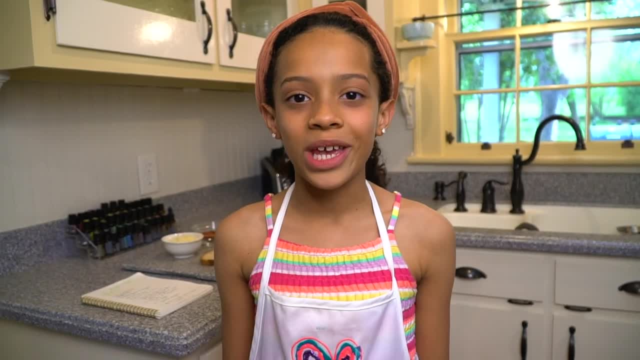 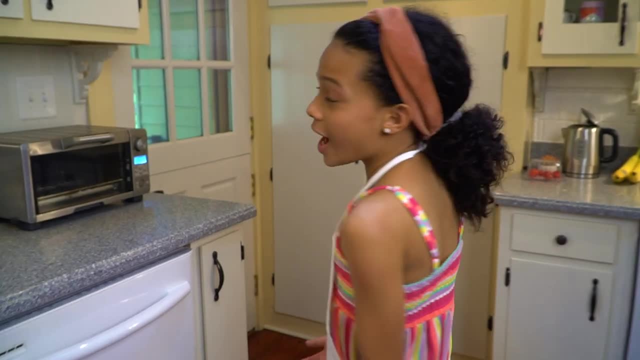 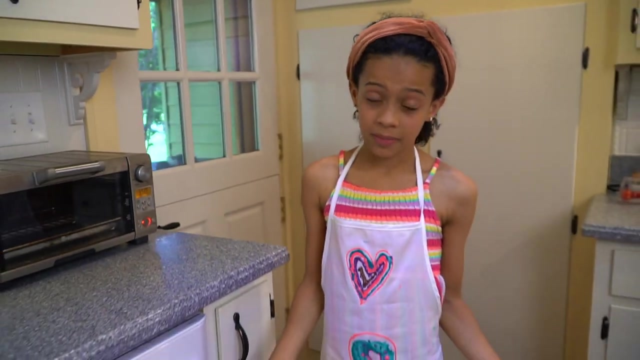 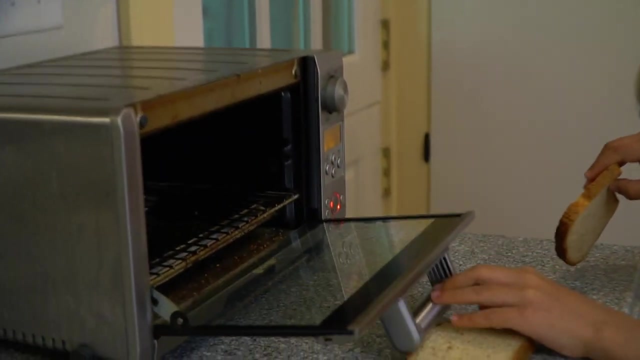 Hey guys, this is Zoey, and welcome to another episode of Kids Cooking with Zoey. This is a fun and easy recipe, but you have to preheat your toaster oven or oven, whichever one you use, and it has to be set to 350.. Now that the oven's preheated, we're going to put the bread inside. 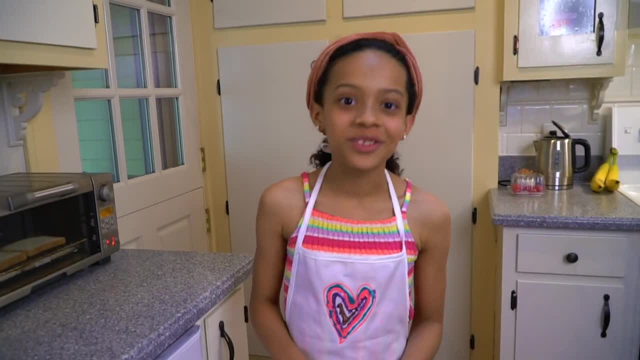 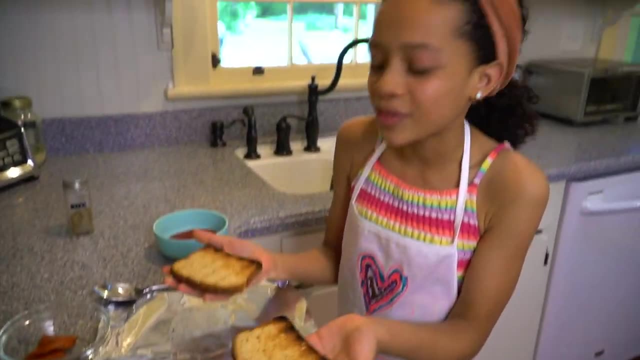 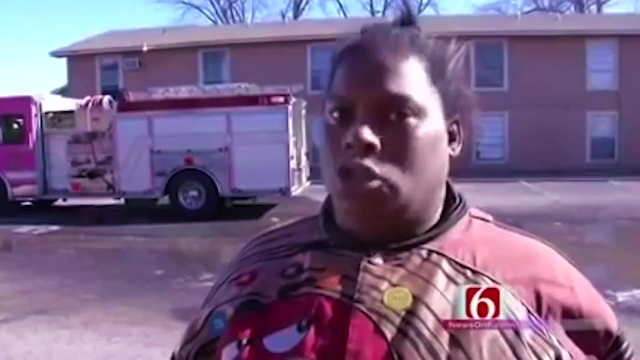 make sure you be careful, don't burn your fingers. now that the bread is toasted, time to make the actual pizza. and it's okay if the bread is a little burnt. all you have to do is flip it over. somebody got burnt. the building is on fire. oh brothers, now i'm gonna add a spoonful of pizza. 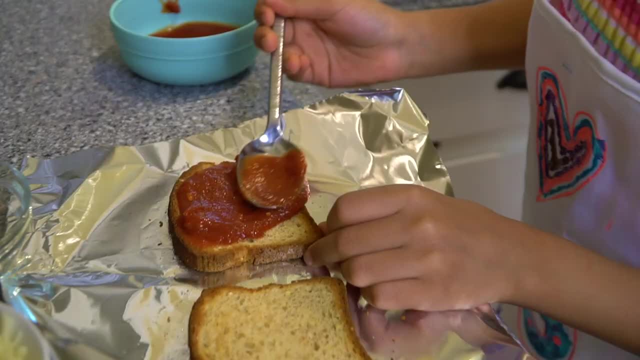 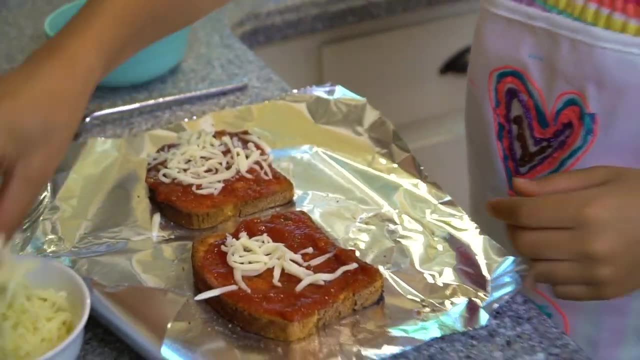 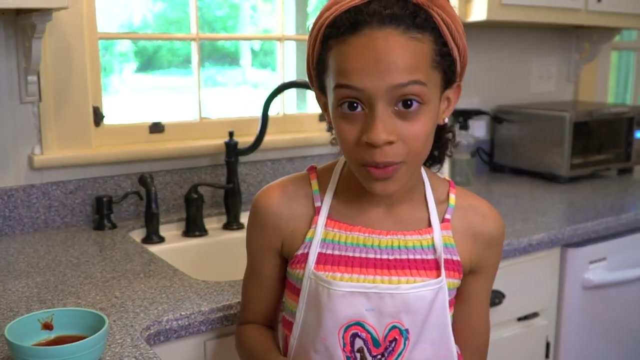 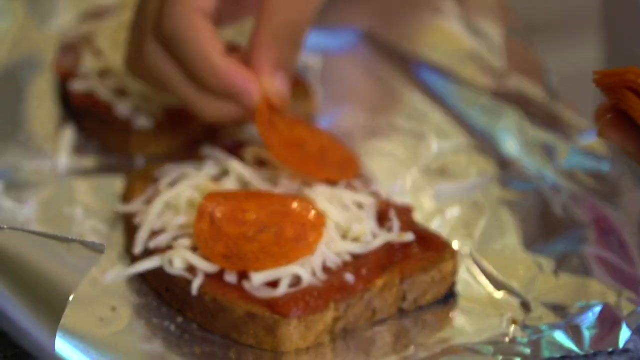 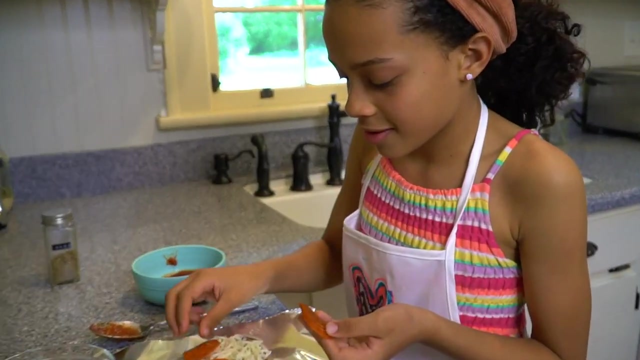 sauce. make sure to spread it with the back. all to the corners. now. we're gonna sprinkle some cheese. i'm gonna add pepperoni, but you can add whatever toppings you want. i'm gonna sprinkle some oregano, you don't? i'm gonna sprinkle some oregano, you don't. 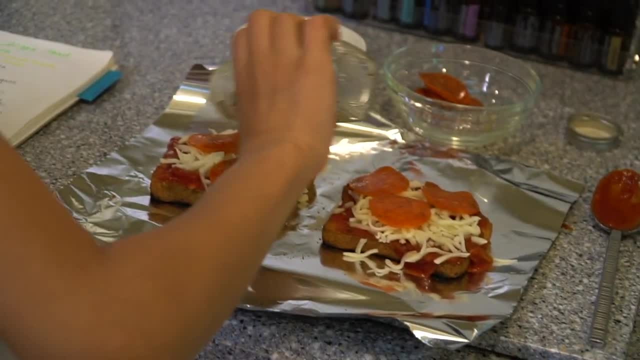 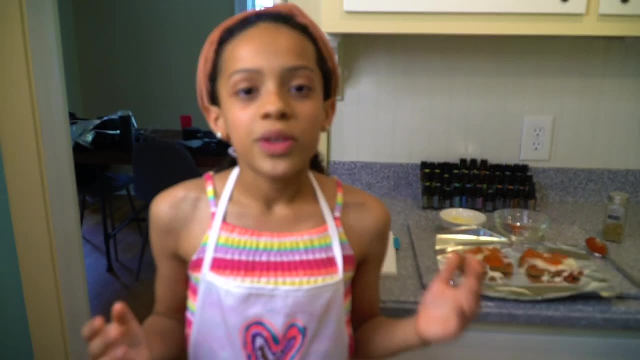 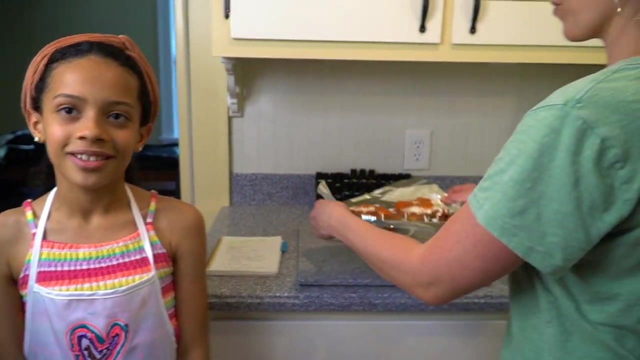 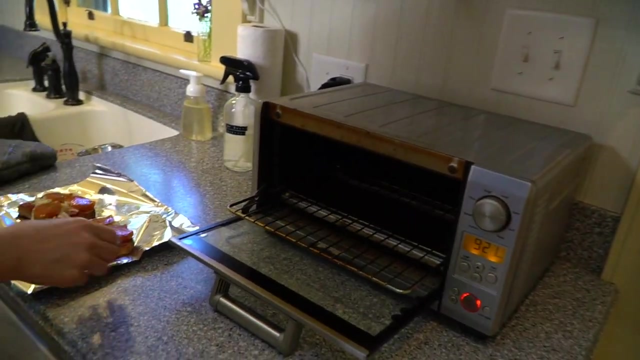 i'm gonna sprinkle some oregano. you don't have to. now that the pizza is done, i'm going to put the pizza toast into the oven, but i'm going to have a little help from my mom, since we don't have a baby. make sure to. 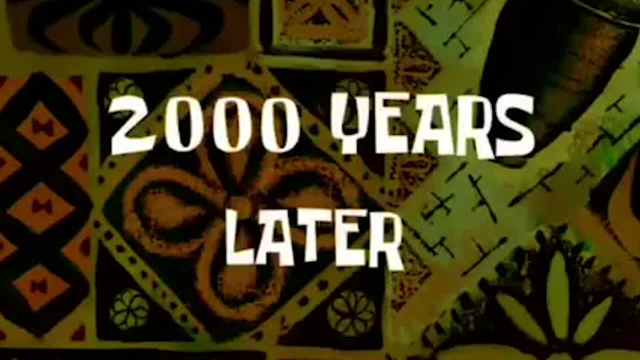 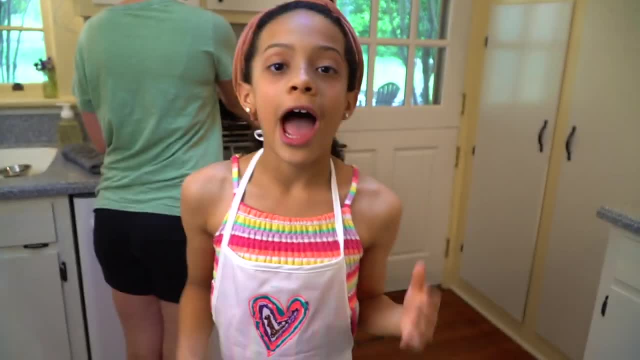 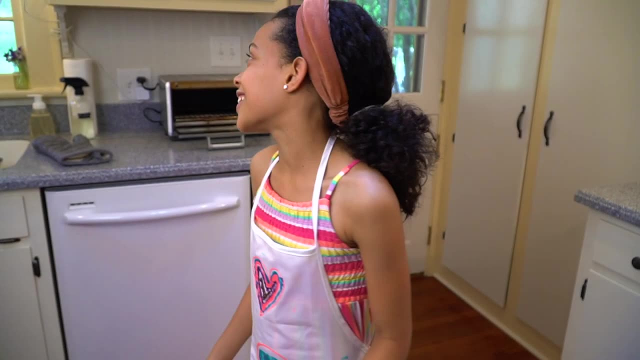 bake it until the cheese is melted. two thousand years later, ours baked for about 10 minutes. now my mom's gonna help me take it out and we're gonna let it cool for about four minutes. alexa set a four minute timer. second timer: four minutes starting.